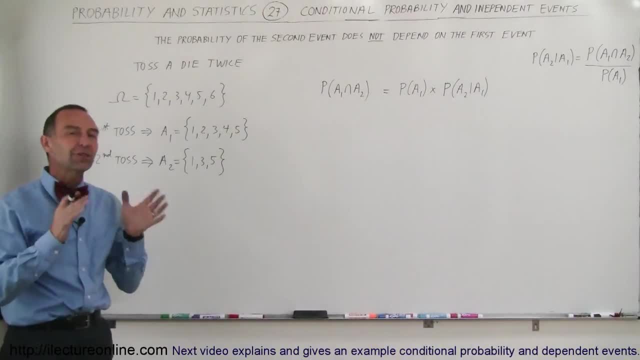 Welcome to iLecture Online. and even though we've seen a few examples of this again, now we're going to go through theory a little bit more and try to relate it to independent events and dependent events in the case of conditional probability. So what we're doing here is looking at conditional 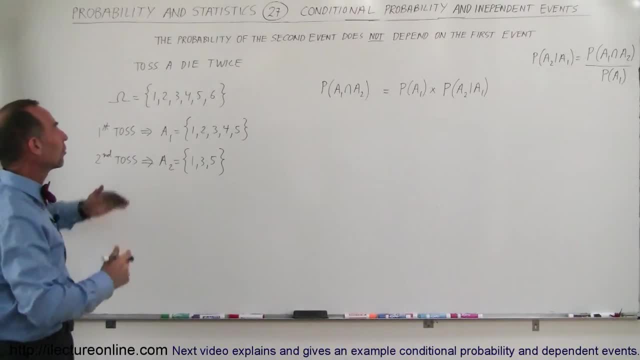 probability with independent events. So there's two events. We're going to toss a die twice The sample space, of course, all the numbers on the die- And the first toss the event is a number less than six. The second event is an odd number. So here what we're trying to find is the 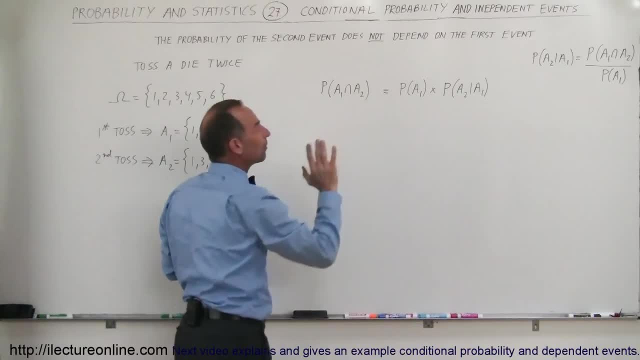 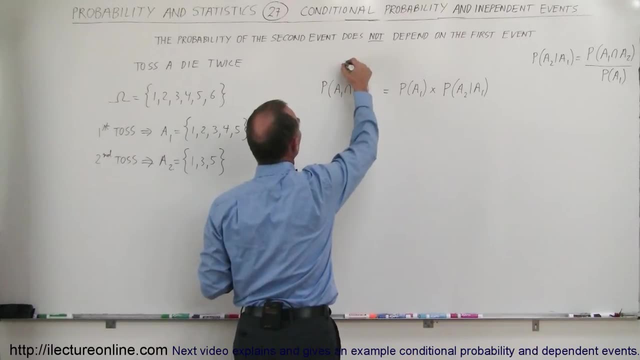 probability of a1 intersected with a2, but a better way to look at it is the probability that event 1 and event 2 will- or a1 and a2, will occur. So let's use the word and here and so the probability. 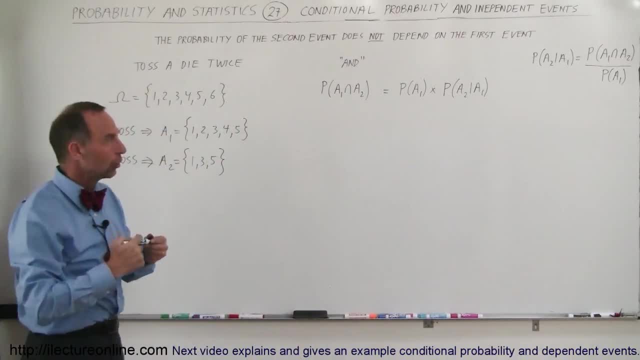 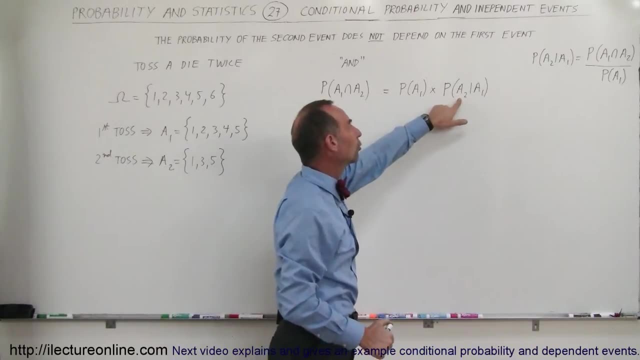 that event a1 and event a2 will occur, and it's equal to the probability that event a1 will occur multiplied by the probability that event a1 and event a2 will occur, times the probability that A2 will occur dependent on event A1.. Now here where 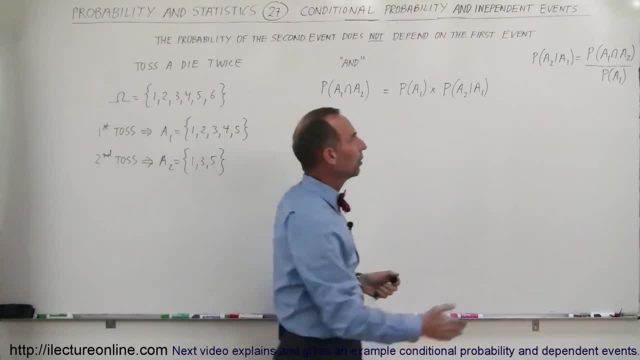 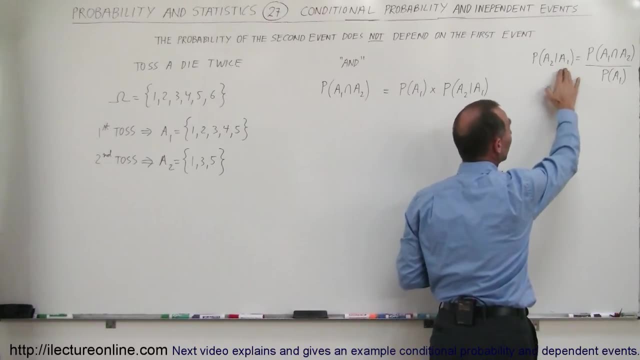 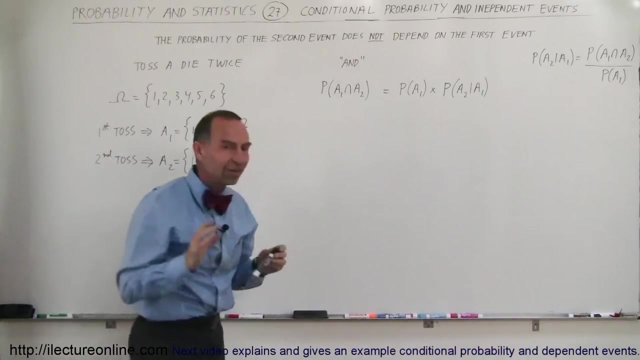 this came from what came from the dependent formula. the probability that A2 will occur, and taken into account that A1 has occurred, is equal to the probability of A1 and A2 divided by the probability of A1.. Now, what's a little? 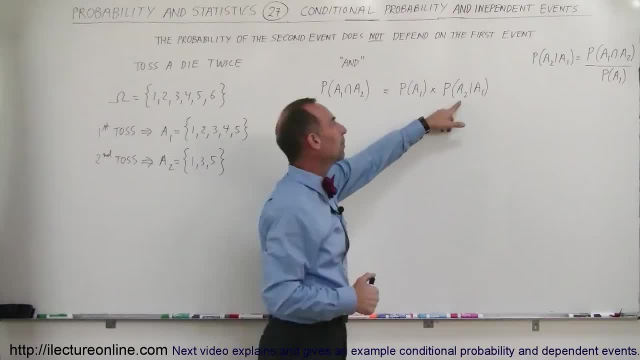 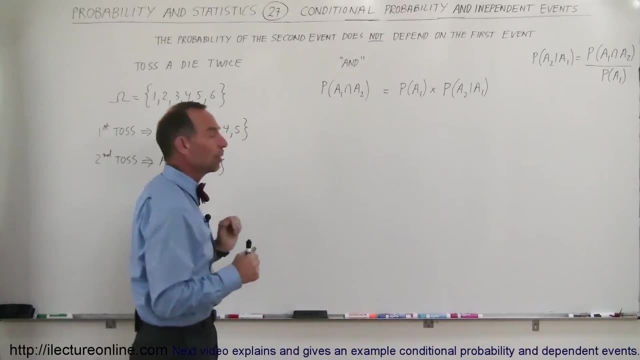 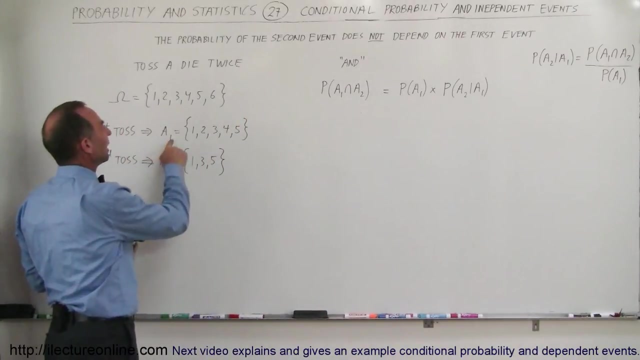 bit different here is that the probability of A2 dependent upon event A1 happen occurred may not really have independence. So let's look at the example right here We're going to toss the die twice. So what is the probability that the first event has occurred and the first event is a number less than six? 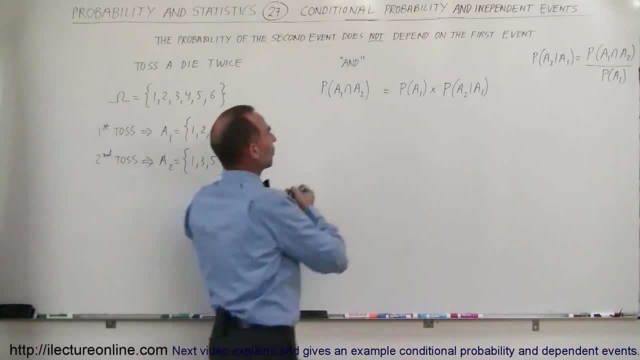 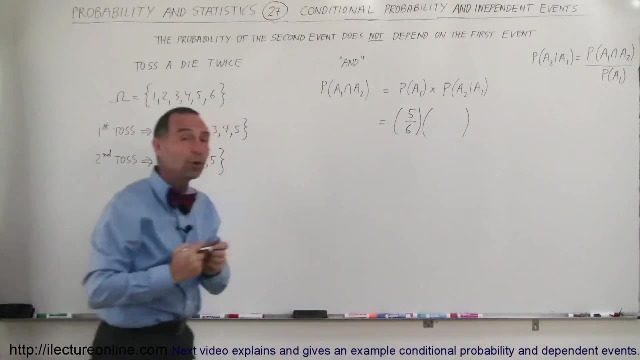 so that's the probability- is 5 divided by 6. in this case, This will be equal to 5 divided by 6.. Now we're going to multiply that times the probability that event 2 will occur, but it depends upon event a1 having occurred. but the fact that we 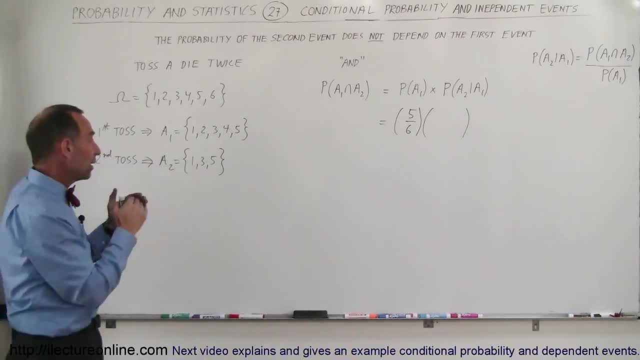 toss it a second time, and that we're looking for an odd number has really nothing to do with what happened in the first toss. it's completely independent on the first event. so therefore a2 will go on it regardless of what has happened in a1, and so therefore the probability of a2 occurring is simply.